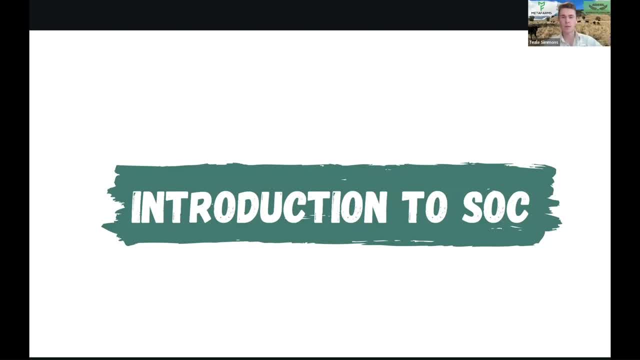 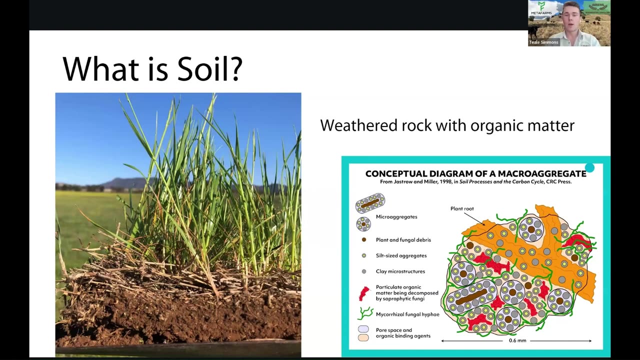 So we're going to start off with an introduction to SOC, But first let's consider what soil is actually like. What is soil? And simply, soil is weathered down, rock, and so we have volcanic activity which produces a bunch of different type of rocks. Over time, that rock is going to break. 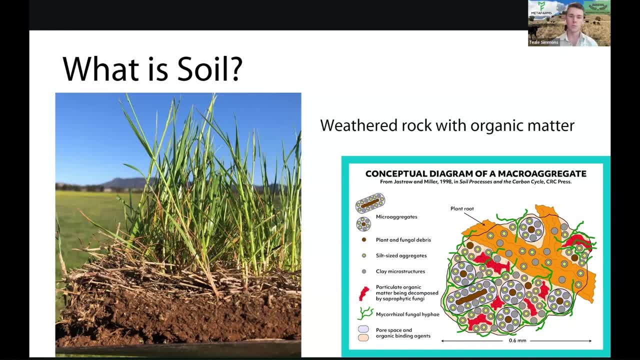 apart and slowly weather down into our clay, silt and sand pieces. Now I define that not as soil but as dirt. And so if you, if you read dirt to soil by Gabe Brown, essentially the part that makes soil turning dirt turn into soil is the organic matter or the life component in between the or in dirt. 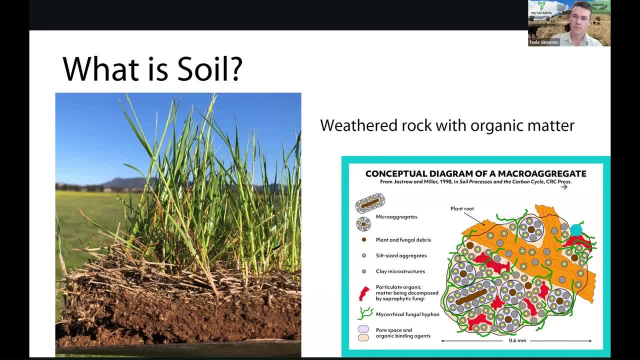 really, And so if you have a look down here at this diagram of a macro aggregate, which is a clump of soil, You'll notice that we have. we have all our mineral components, or clay, silt, sand, but it will also have all of this organic matter binding it all together. We also have our mycorrhizal fungi. 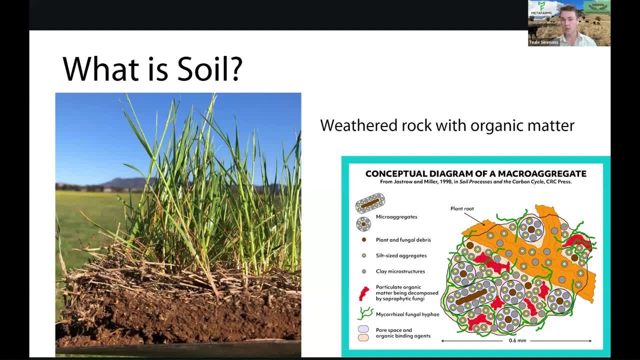 binding all together. Even in inside of that we'll have bacteria and all different type of other microbes, And we have our plant roots, And so, really, our soil is a is a teeming um piece of matter full of life, And so the most important part to take away from this is that 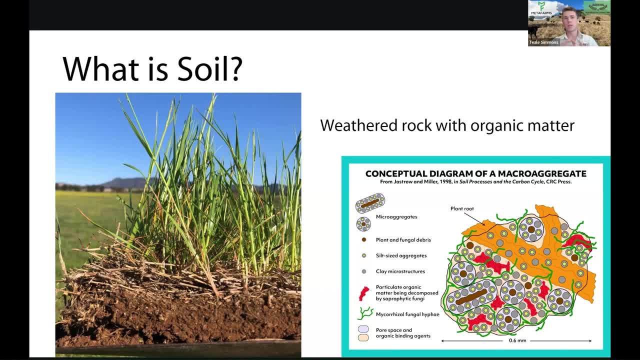 soil is more such. it is a biological um medium as much as anything, And it's very important to treat soil as a biological um medium rather than just thinking it is simply a um unliving piece of dirt. So yeah, there we go, We've got. 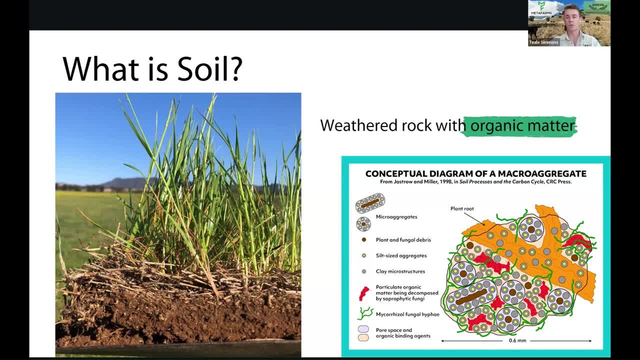 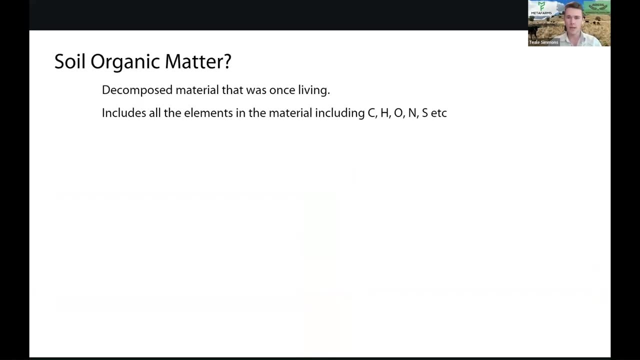 the organic matter in between our weathered rock is truly what makes our soil So soil, organic carbon or soil organic matter more specifically, is simply decomposed material that was once living. So when we hear organic, it's not saying you know something? certified organic in a. 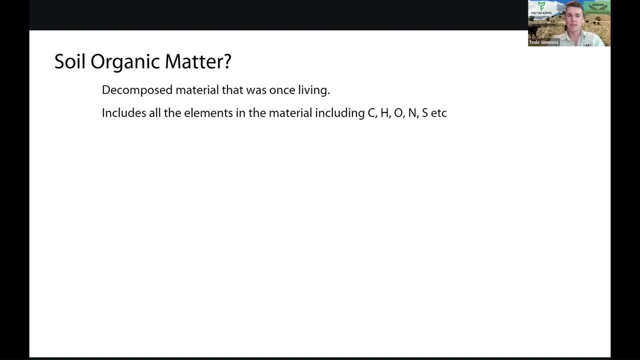 food production sense. But organic um means it has a carbon component to it, So it was once living and so this includes all elements in that material, such as our carbon, but also hydrogen oxygen, nitrogen, sulfur and all these other different nutrients and elements and minerals. 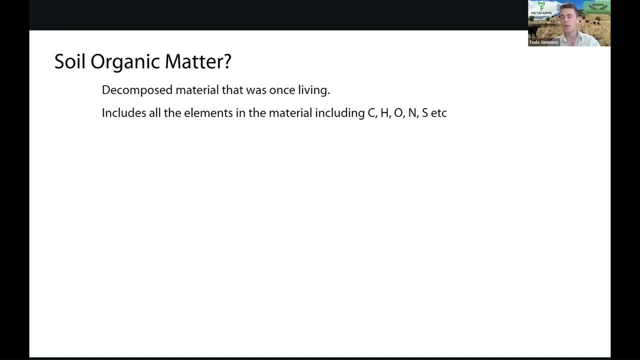 that are in that component. so if you think of like a leaf, there's such things in that leaf, but all of that combined, once it's decomposed, is our soil organic matter. so what's the difference between soil organic matter and SOC? well, soil organic carbon is a carbon component in soil. 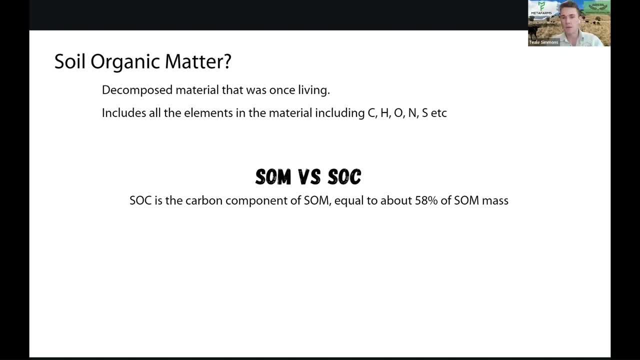 organic matter, and that's a. it's about 58 percent of the soil organic matter mass, and the reason why we look at soil organic carbon and not soil organic matter specifically is that it's much easier to measure soil organic carbon in the lab rather than soil organic matter, and so it's just 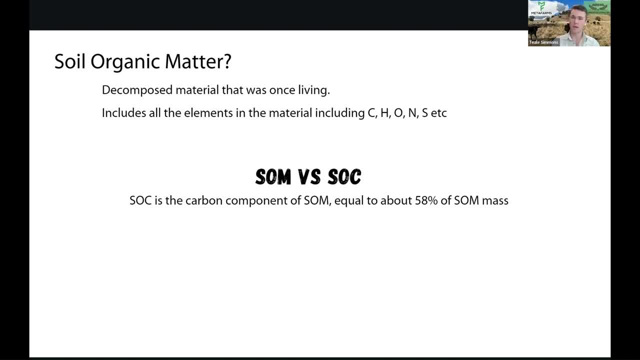 easier, like if you get a, if you get a soil test result back, you'll um, you'll get the soil organic carbon and not so much the soil organic matter. so for that reason it's easy just to talk about soil organic carbon. so what is soil organic carbon? it's the 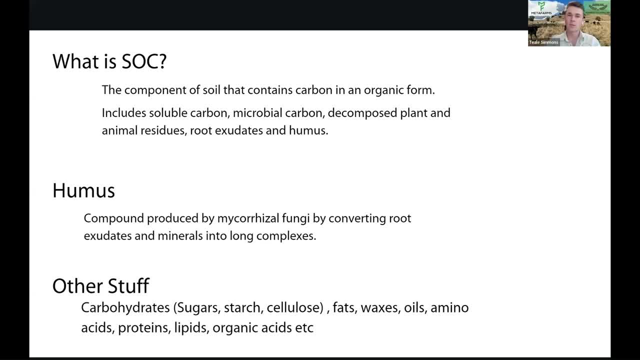 compound uh. it's a component of soil that contains carbon in an organic form. so this includes all of our soluble carbon. so all our sugars and stuff uh. microbial carbons, all the carbon in our microbes. decompose plant and animal residues, so think of manure or decomposing plant material root. 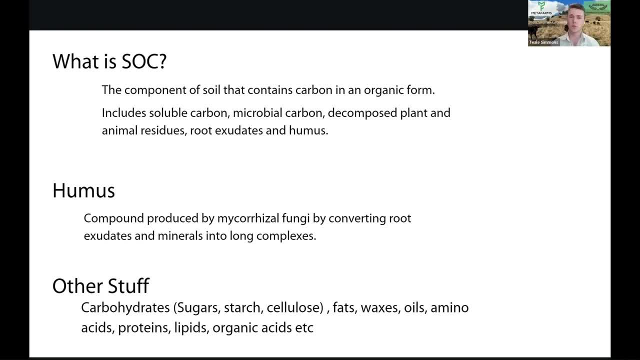 extracts and humus, and so it's important to know that there's really two kind of categories. we can put so organic carbon into, so humus, and then there's other stuff, um, and doesn't really matter what um. I guess the other stuff is because humus makes up 65 to 75 percent off stock, so really it's. 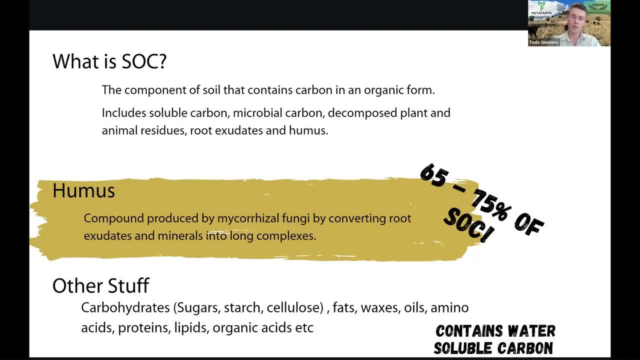 humus that's doing the heavy lifting in our soils and that's a comp as a compound produced by mycorrhizal fungi by converting root extra dates and minerals into these really long complexes. so simply, they're not a simple defined compound, they're really these really long spider web type. 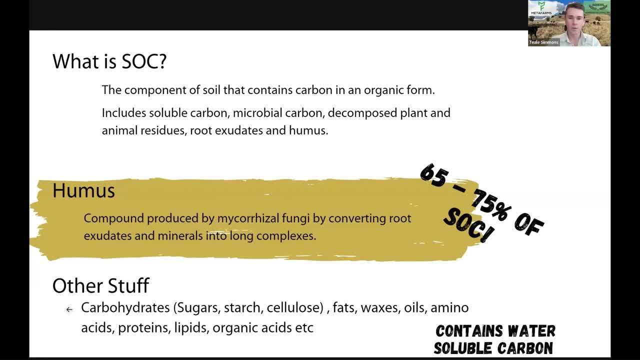 things in in our soil, um, and they're very complex. now our other stuff is going to include um, these compounds which are quite easy to define by chemical formula. so oil, carbohydrates, fats, waxes, oils, amino acids- our pro? um- and proteins, lipids, organic acids, really everything else that has a 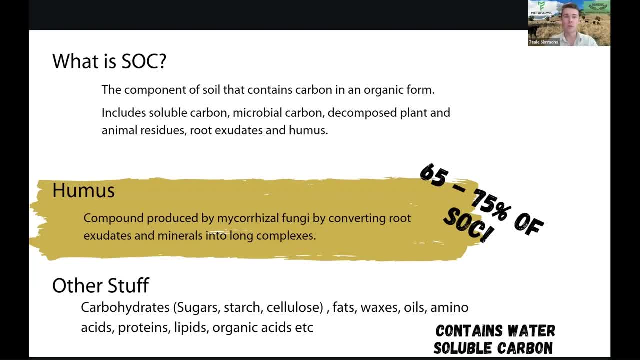 um carbon component to it. now it's also important to know that soil organic carbon isn't um. it doesn't include the mineral um carbon in our soils. so, for example, our carbonites, so calcium carbonite, that although it does have carbon in it, that's not still organic carbon. so it doesn't. it's not. 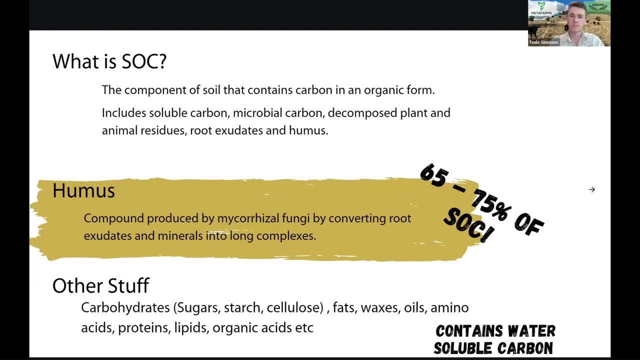 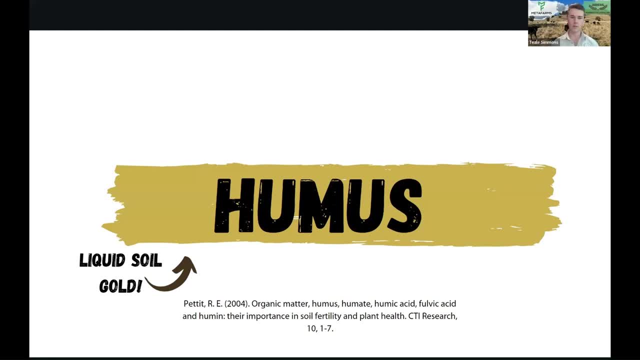 derived from a once living thing, so humus, since it makes up so much of the organic carbon in our soil. I want to touch a bit more on what humus is and what's made up of. and really, as I say, in the corner, there it's, it's literally liquid soil. gold like this stuff, really. 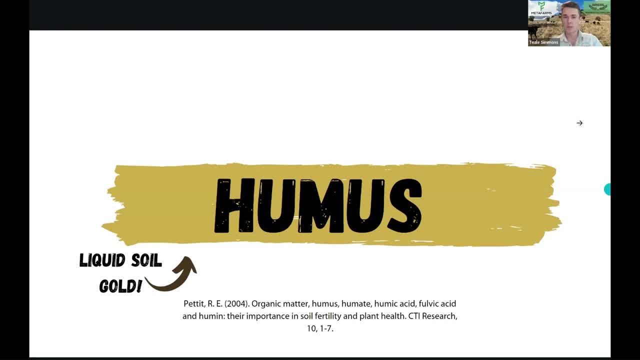 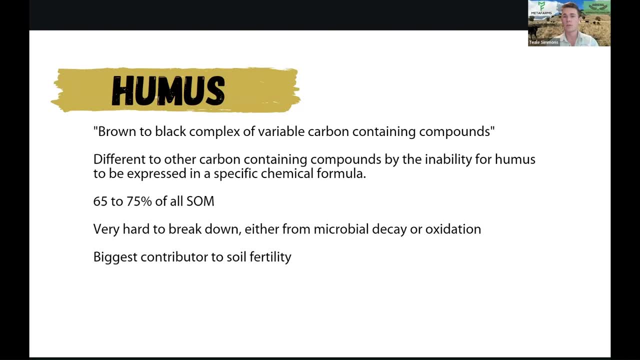 contributes so much to our soil fertility, and we'll touch on that in a bit. so humus humans is a dark to a brown to black complex of variable carbon containing uh compounds. yeah, so so it's. it's carbon containing compounds by the inability for humus to be expressed by a specific chemical. 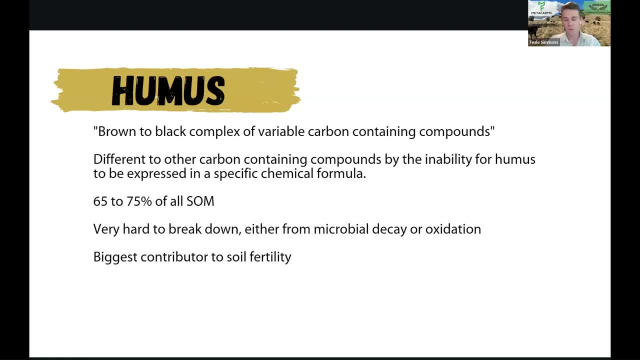 formula. so if you look at um glucose, for example, that has a very, it's a fixed chemical formula. everything that has a chemical formula is glucose. humus doesn't act like that it's. it's a complex, so things can keep being added to it. humus in one, you know, plot might be different to a plot in another. 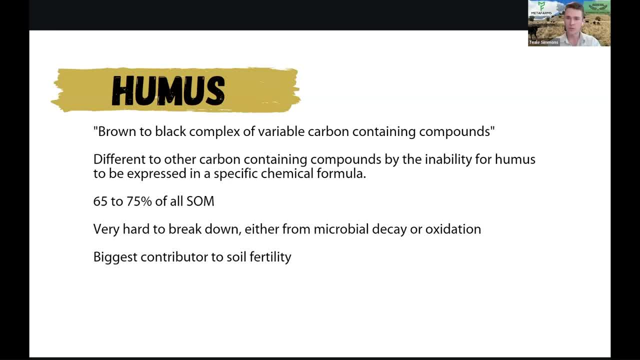 um. so for that reason, it is very difficult to define what humus is specifically. um, it makes up 65 to 75 of all our song, as I said before, and so, for this reason, that's why we really want to focus on it. the other reason why we really want to focus on 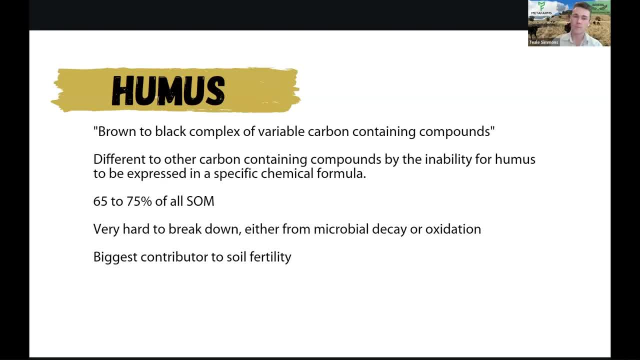 it is that it's very hard to break down um, both from microbial decay, so microbes can't really eat it as um readily compared to our other sources, and it's very hard to oxidize, which is essentially burning something without a flame um and again, it's our biggest contributor to soil health. 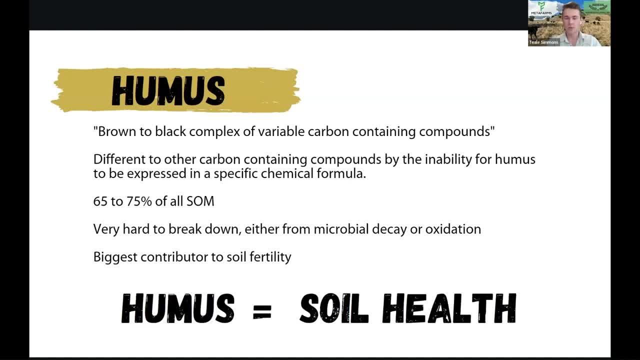 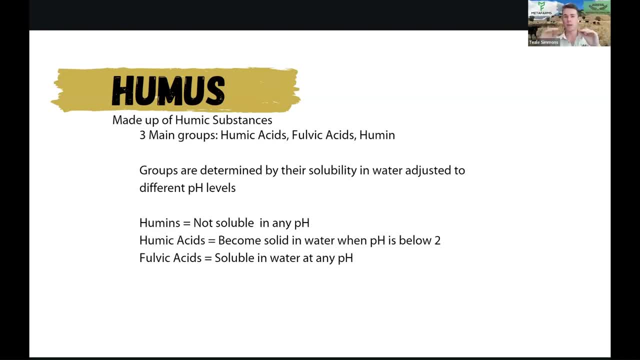 so humus is equal to soil health. so the more we can build, the healthier our soils are going to be. so humus is, I guess, the the overarching category. within that we have humic substances, and so there's three different type of humic substances, that's humic acid, phobic acid and human. so these groups. 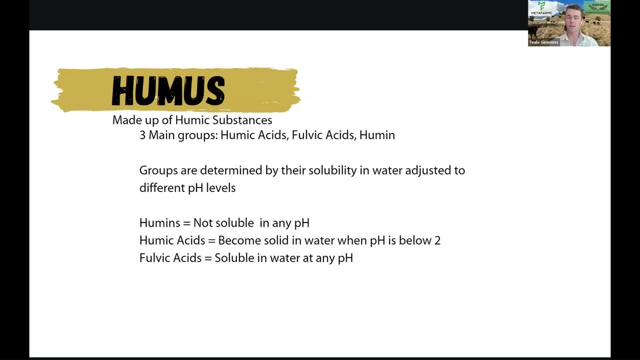 are determined by their solubility in water adjusted to different pH level. um and because, as I said before, we we don't have a specific chemical formula for humus, um it's it's hard to separate our groups by their chemical formulas, and so that's why we're looking. 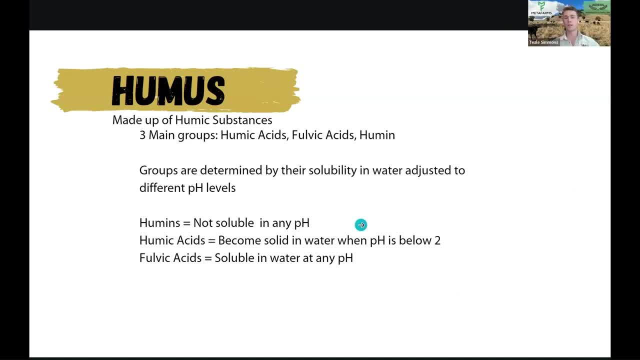 at it at a pH level, and so humans, they're not soluble at any pH. so they're just not soluble. uh, humic acids become soluble in water when pH drops below too, so when these things are really a uh, they become- oh sorry, they become- solid in water, and fulvic acids are soluble in water at. 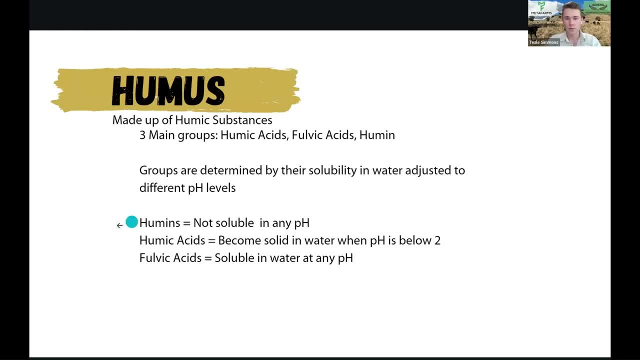 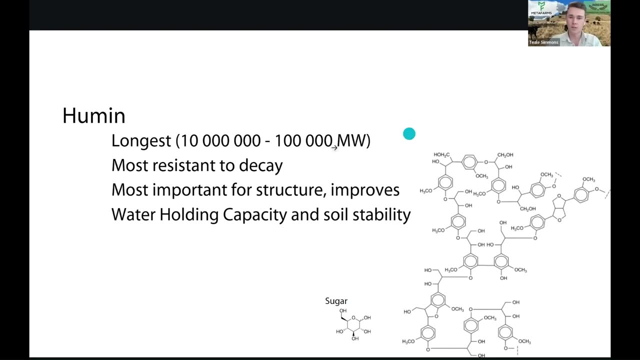 any ph and so, when you think about it, not soluble at all soluble. and then somewhere in the middle are humic acids, human. so this is our largest um, humic substance, um, when we look at this. so this is a molecular weight, um, just for the easiest and most simple way to explain it. just look at: 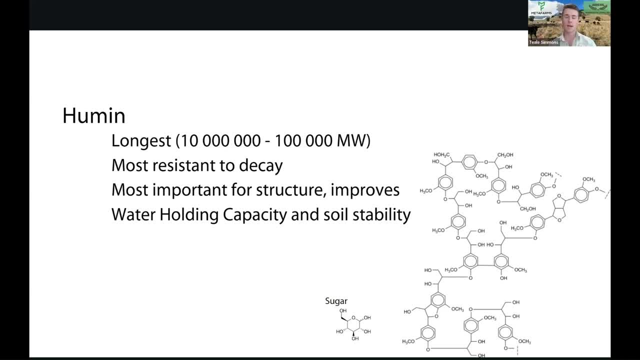 the difference between human fulvic acid and humic. um, yeah, humic acid, um, these weights don't really matter too much, but think of it as a relative difference. but essentially these are massive compounds. when we look at this diagram here and compare it to sugar, now, sugar as itself is a 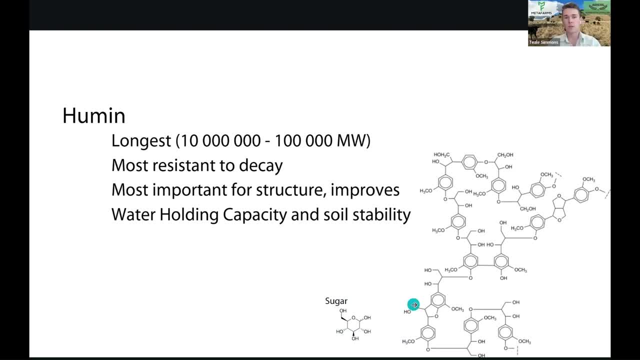 pretty large compound. these things are just massive in our soil, and so, for for that reason, they make up a lot of um structural integrity within our soil, and so that's its main function. um this particular humic substance, it really does improve our soil structure and also improves the water holding. 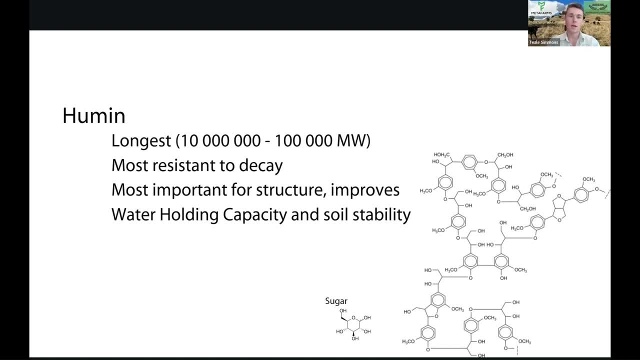 capacity and soil stability. so when you think of uh human, think of it as like the building infrastructure in our soil. it really holds. it's also the most resistant to decay out of all our humic substances. next one is humic um acid, so this is the one in the middle. now this is pretty good because it it combines with clay to 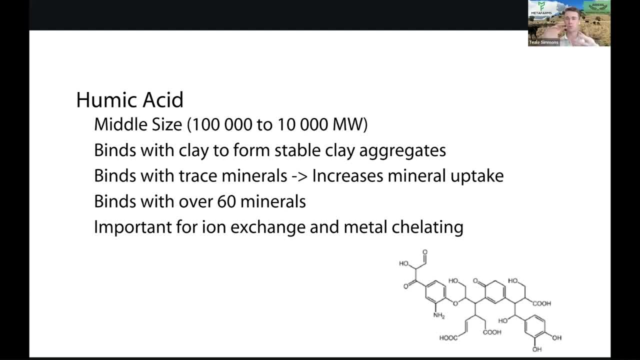 form stable clay aggregates. so if you think about humic acid forms, it binds to the clay particles, which is our smallest particles, and then we have our uh human, which structures everything around that. now it has um these active sites on the compound. so you can see um a lot of the times. 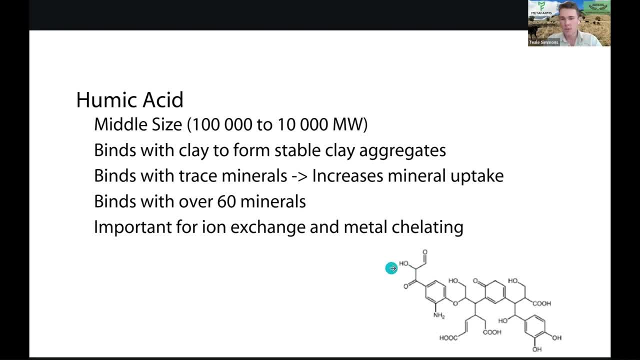 when you have an oxygen that's um, an active site, so we've got a um alcohol group, well, some of these double bond oxygens. so usually at these sites there's a chemical difference, so there's a chemical charge on these points, which means it can, it can bind to trace. 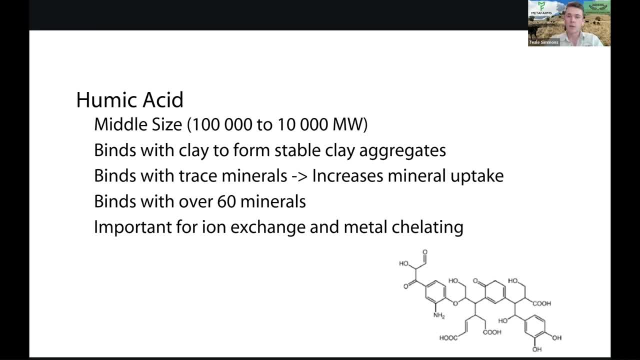 minerals or just minerals in general, and so this allows an increase in mineral uptake, so a lot of plants actually prefer to absorb minerals in these complexes, and humic acid can actually combine with over six percent of the Sleeping and Flowing Bonds mit 60 different minerals, and so this is really important when we're trying to increase the. 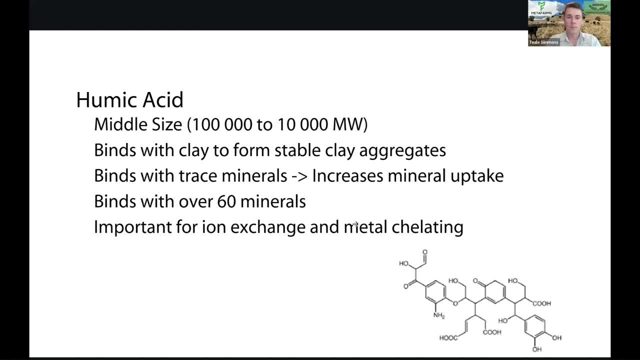 absorption of minerals by our plants. Now, the other big component of this is that it has a really big implication for ion exchange. So if we want to increase our cation exchange capacity- which is essentially how big our bank account is- in our soil to hold on to ions or cations, 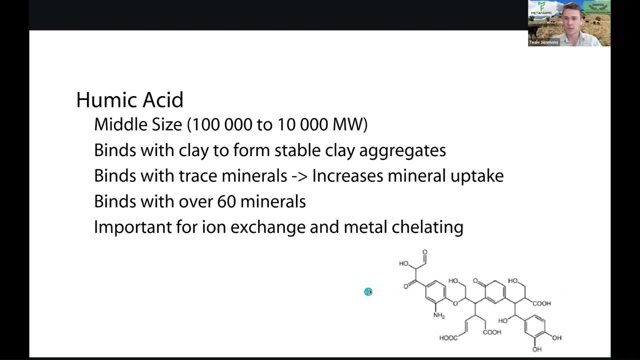 we want a lot more active sites in our soil, and so humic acid gives us these active sites in our soil for these minerals to cling on to. So it's really important for that, and we'll touch on that a bit later. and it's also important for mineral chelating, which I've touched on before We'll get. 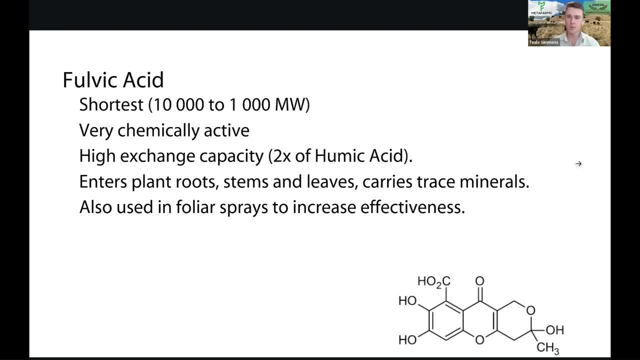 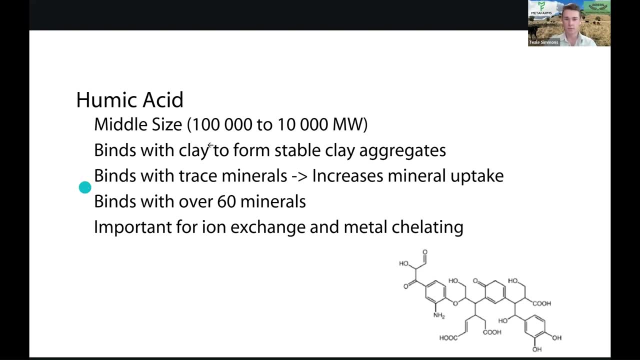 into a lot more of this in a bit. Fulvic acid: Now, fulvic acid is the shortest of the lot. so if we compare fulvic acid, which is fulvic acid, which is 10,000 to 1,000 molecular weight, to 100,000,, 10,000 for humic acid, and then human, we got. 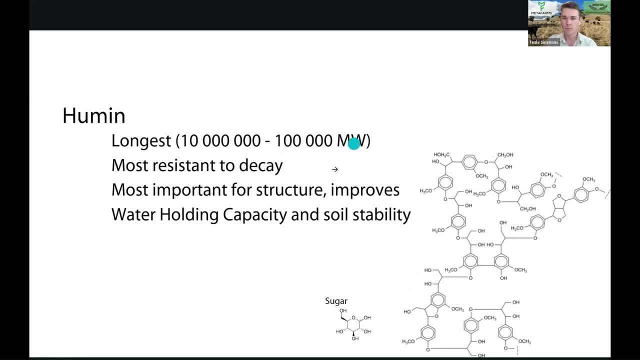 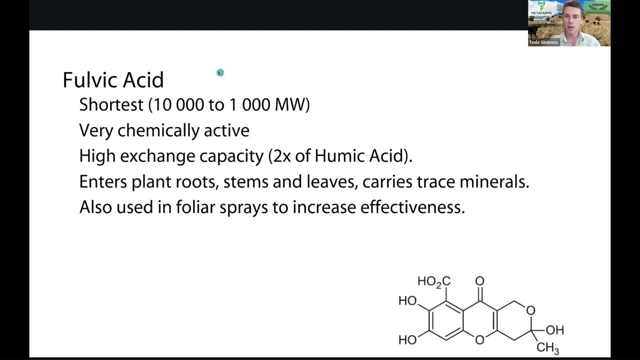 10 million to 100,000. So you can really see the difference in the size of these compounds. Fulvic acid is the most chemically active of all our humic substances. It has a really high ion exchange capacity. so it's almost twice the has twice the capacity. 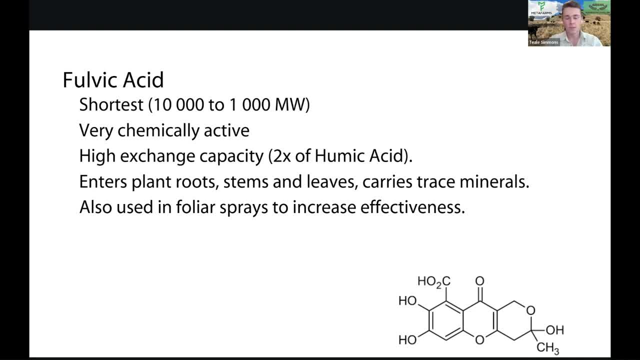 of our humic acid. It's so small it can actually enter into plant roots, stems and leaves and carry the trace mineral with the compound, And so typically this can be used in foliar sprays to increase the effectiveness of the foliar spray, but also in our soil it's. 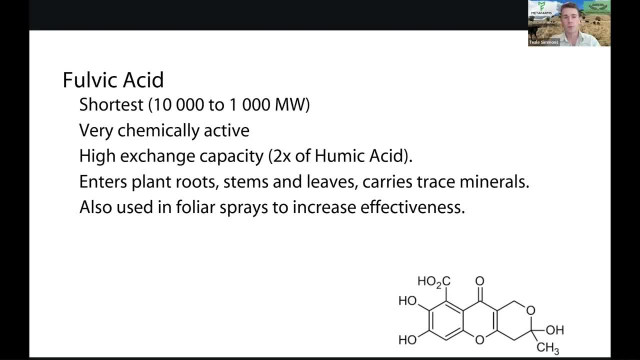 going to increase the effectiveness of the uptake of nutrients into our plant, And so that's really important. if we, you know, want to increase our fertilizer use efficiency, A lot more of our fertilizer will be going into our plant. And yeah, that's. that's an example of the molecule. 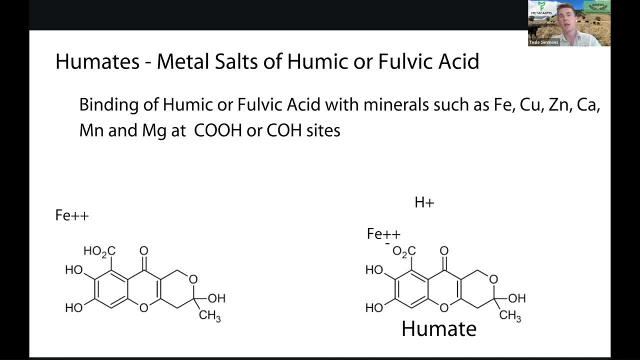 So there's another group of humic substances. it's not a humic substance in, I guess, a particular way, but more so it's a combination of a humic substance with a metal or a mineral, And so these, these are humates. so humates are metals of salts or metal salts of humic or fulvic acid. 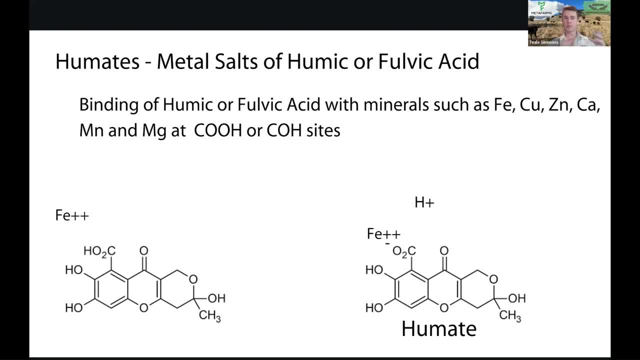 so it binds. it's a binding of humic and fulvic acid with minerals such as iron, copper, zinc, calcium, manganese and magnesium at these, at these sites, so our um uh, their carboxylic acid sites and our alcohol sites, and so what happens, say, for example, is we have our um iron here. so 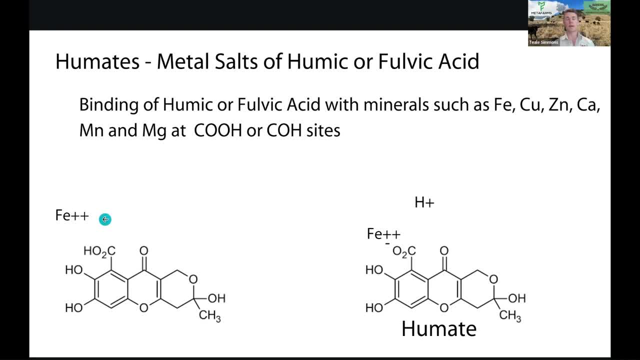 it is more um energetically favorable for this iron to be attached to this um fulvic acid, and the way that this occurs is that this um hydrogen iron here basically gets removed off of the compound and which makes the the compound itself have a negative charge. now, negative and positive things attract, and so 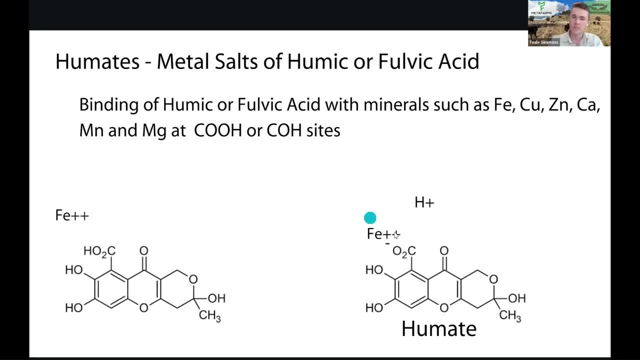 this um iron compound here will attract itself to the fulvic acid and therefore forming a um humate. now, this is this is actually what gets absorbed into the plant. so this whole thing will get absorbed into the plant, um, which improves the efficiency of um, the absorption and the use. 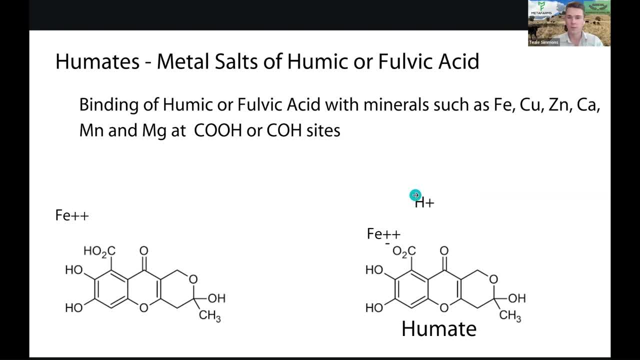 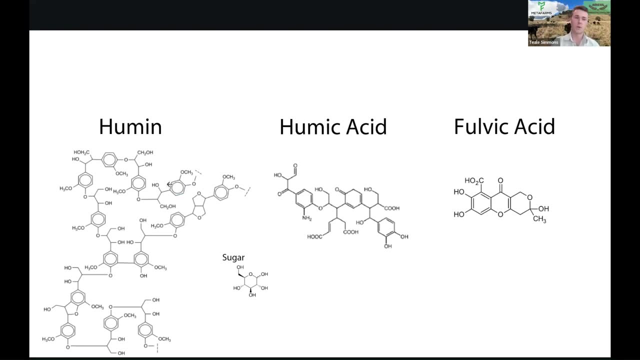 and so this is one way that we can um increase absorption but also cling on to a lot of these minerals and make them more available in our soil. so here we. here we go again. here are our three um uh humic substances. we've got human, so quite a big compound. humic acid and fulvic acid compared. 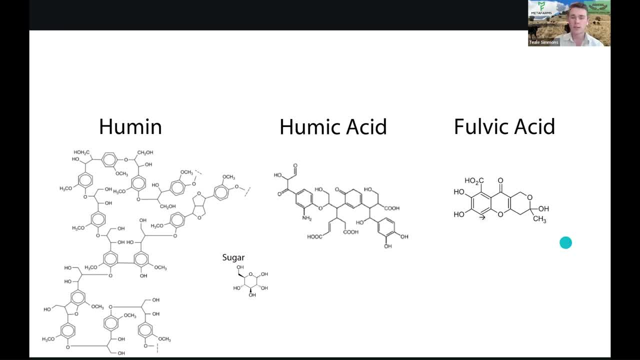 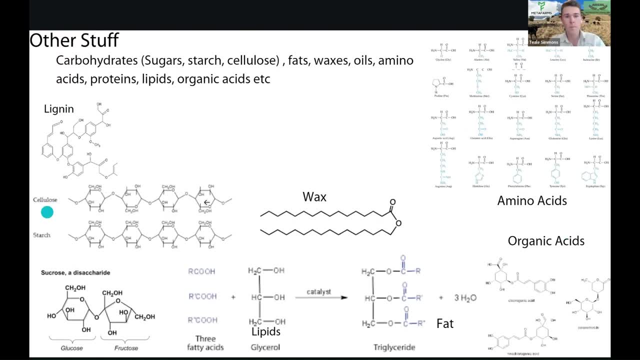 to sugar. so it's important to also talk about the other stuff. so we've got uh carbohydrates, which are, uh, these ones here, so cellulose and starch, um, so they're, they're a bit more of their complex um carbohydrates. we have our simple sugars, which are um glucose here. so this single one we have um. 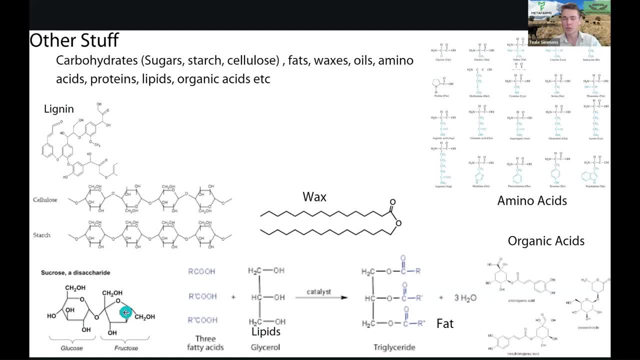 fructose as well. they're examples of reducing sugars. so very simple sugars or monosaccharides. then if we have both of them together, that's a disaccharide, so two together. this is not too much important, um, but it's. i guess it's just important to know that there's a lot of different. 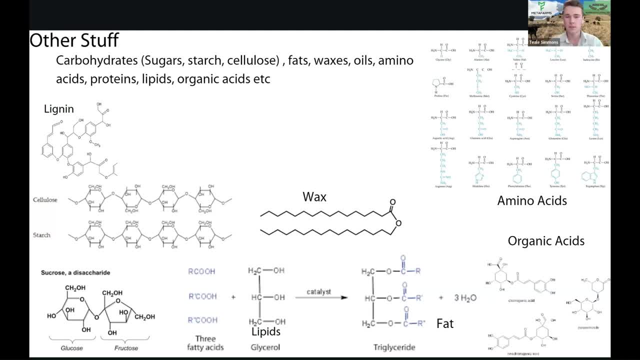 other things in our soil that's still important um, and all makes up um soil: organic carbon. also have our fats um, which are here, so triglyceride, but we have our um oils, um, where the oils are here and are there lipids. we have uh fatty acids, we have our waxes, we have our amino acids. 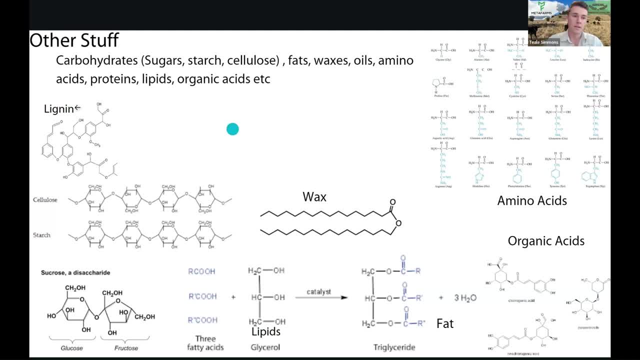 which are quite important. organic acids, um uh, ligulin, which is uh a hard to break down carbohydrate, typically in plants, and so all of those together make up all the other stuff, and typically we get this from the decomposition pathway. so when we add in our human, we get soil, organic matter, and so all of this, think of all of these things in our soil. 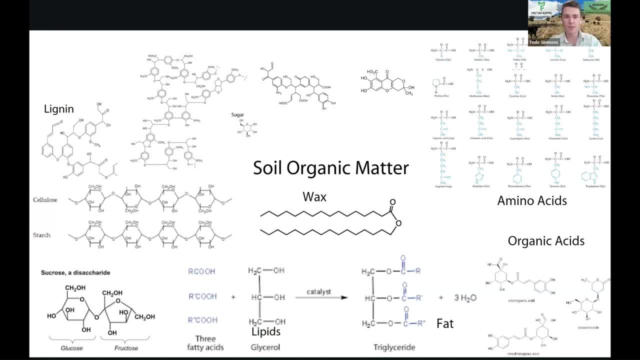 um, or doing different things and, um, i guess, reacting with each other, um, and being used by microbes and and all that. so all this together is soil, organic matter.